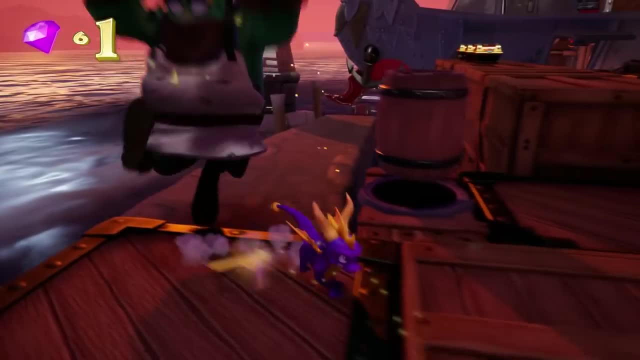 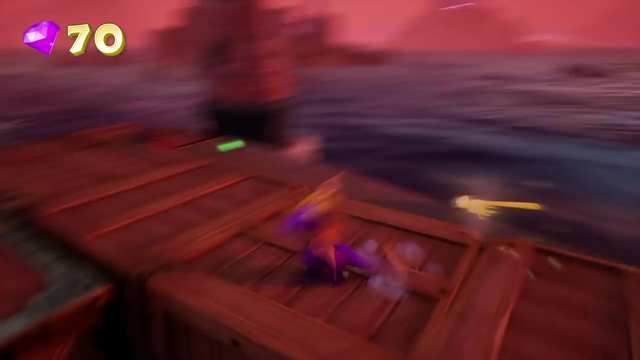 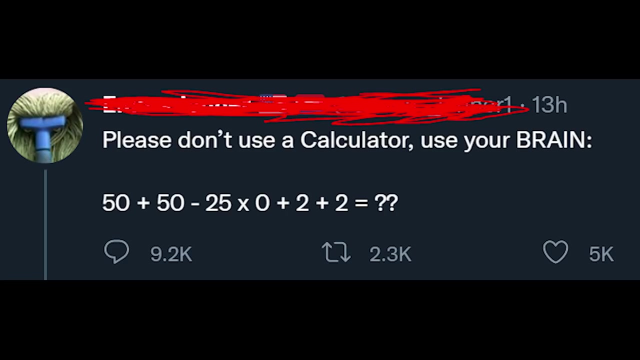 let's put it into a calculator. So if you enter an equation into a calculator, it will give you the objectively correct and one and only answer. Any differences is because of how the equation is written, or something like that, But this particular equation that you've shown us, there is only one answer, yet people are getting thousands. 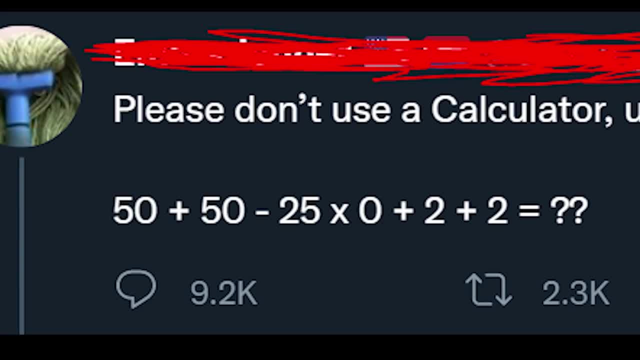 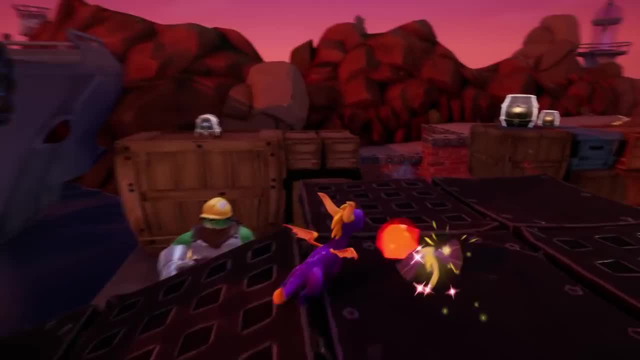 So let's just take a look at the equation: 50 plus 50 minus 25 times 0 plus 2 plus 2 is equal to question mark. Honestly, seems like a super simple equation. I mean, if you know PEMDAS. 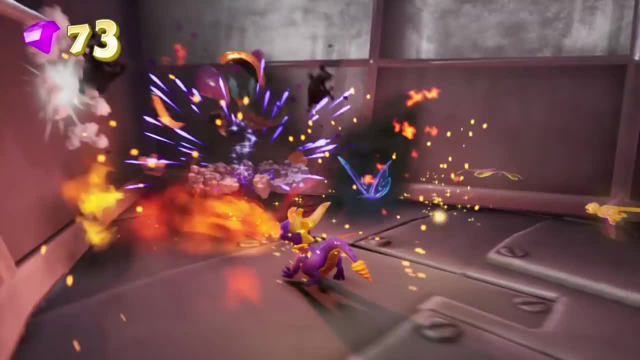 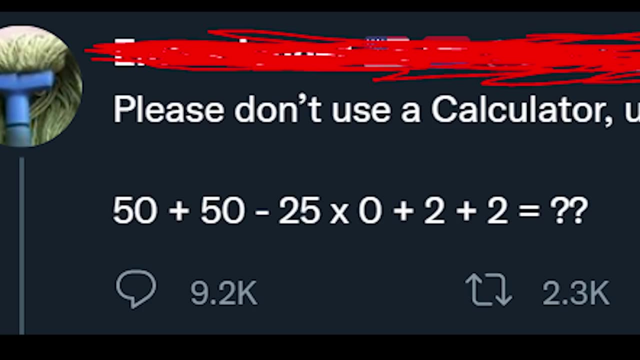 or BODEMAS or whatever the hell. the order of operations: multiplication goes first, so it's minus 25 times 0, which is 0. And then you just complete the addition 50 plus 50 plus 0 plus 2 plus 2,, which is 104.. 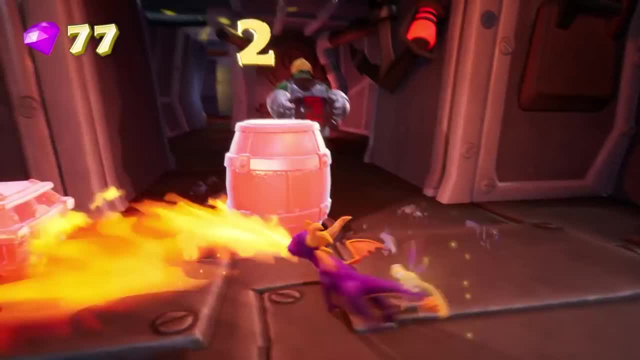 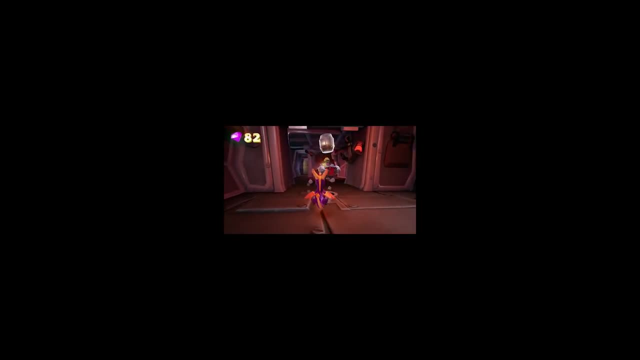 Let me just settle the debate here and forever. The only one objectively correct answer is 104.. If you get anything else, you simply are a lower life form. So let's start with Professor Moron here. okay, He says, okay, class. 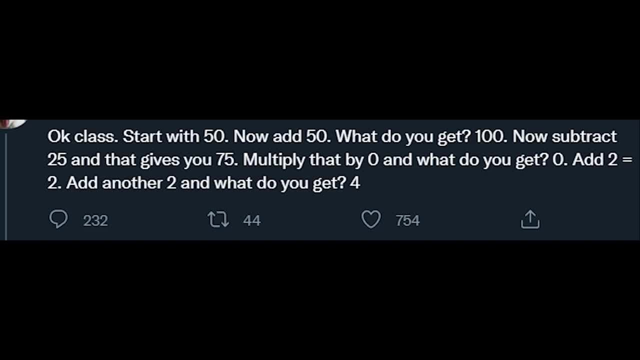 start with 50.. Now add 50. What do you get 100.. Now subtract 25.. That gives you 75.. Multiply that by 0.. What do you get 0.. Add 2, and you get 2.. Add another 2, and what do you get 4.. 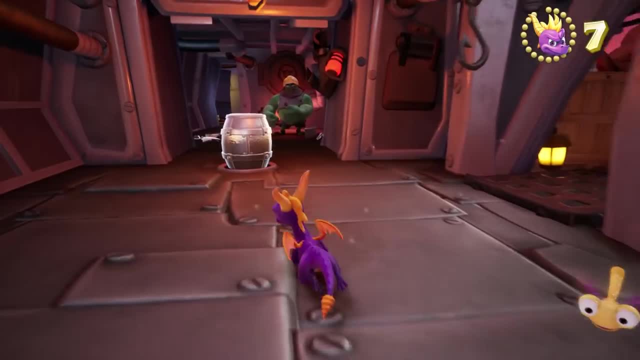 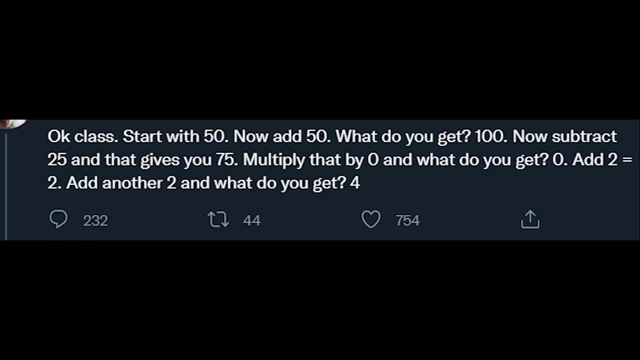 This man has, like put the pen down, thrown the marker at the board, just been like boom served. I've got it right. The answer is 4.. Now this guy actually messed up line 1. He did get it right that 50 plus 50 is 100, but you do not start with that. 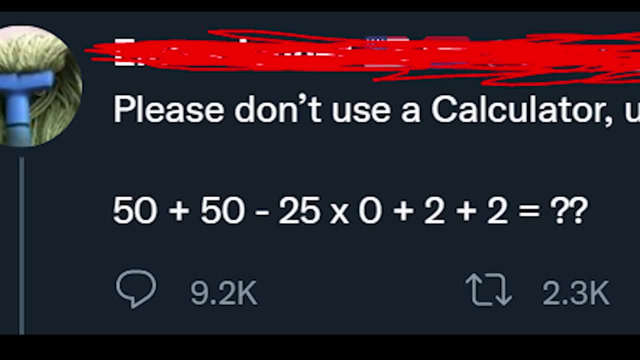 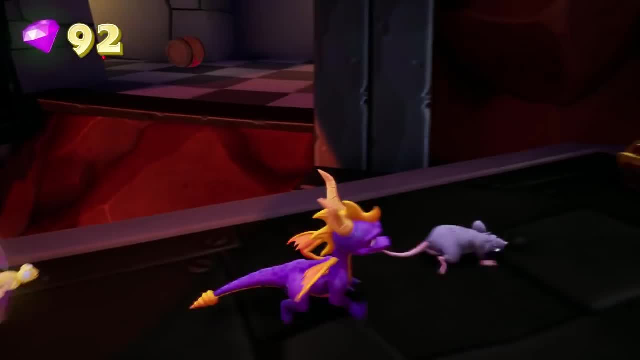 In this equation, you have to start with multiplication. That's just a general math rule, And I know some people will immediately argue: well, uh, there's no brackets, therefore you go left to right. No, that's not how it works. 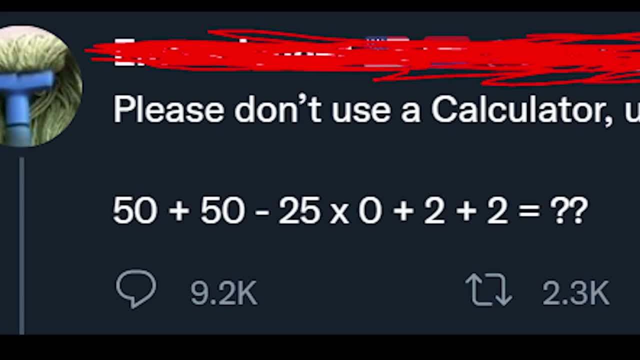 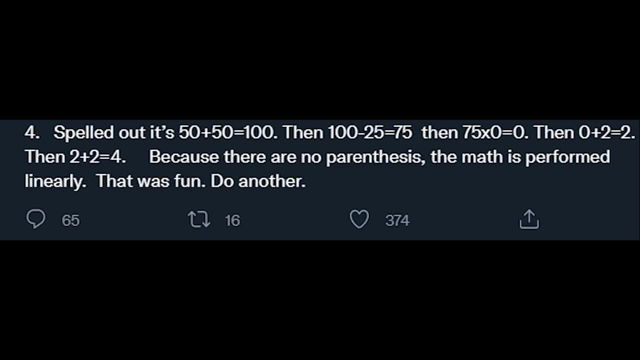 There's implicit brackets when there's a difference in signs. If I were to put brackets around this equation, the first brackets would automatically go to the multiplication sign. Now here we have another individual who rivals the IQ of Albert Einstein and Deji, himself: 184 IQ. 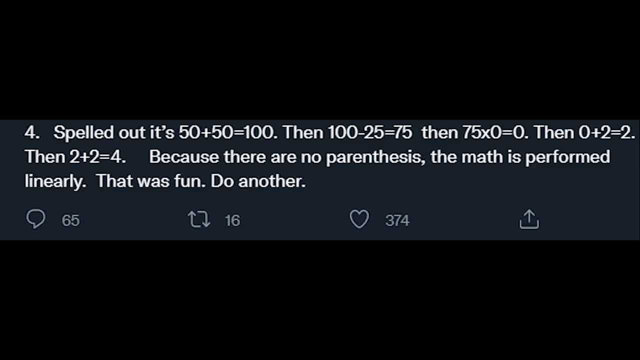 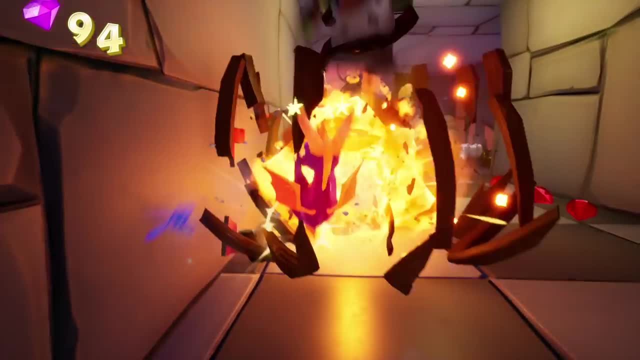 Because there is no parenthesis, the math is performed linearly. That was fun. Do another, No, no, no, don't do another, You're still stuck on this one moron. This guy's the type of guy to do an exam and just be like, oh, okay, okay. 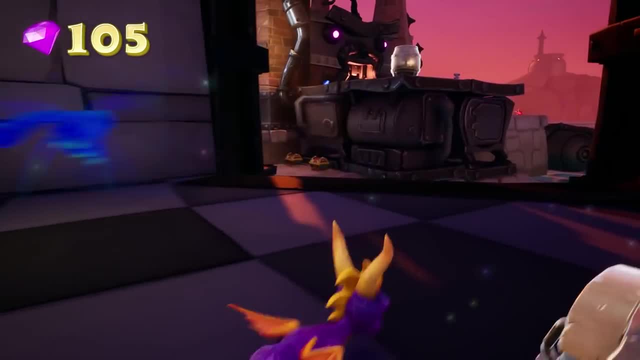 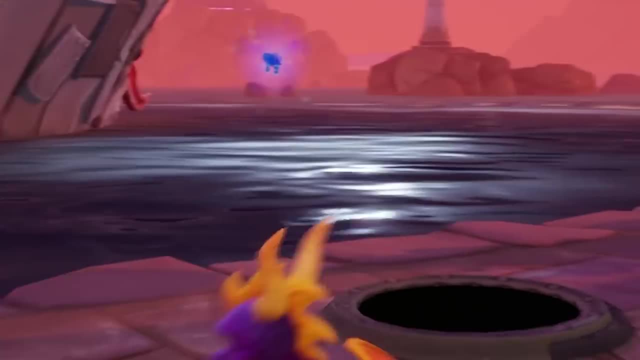 I finished this question already. Oh, I'm already on question 2.. Oh, you're still on question 1? What an idiot, bro. And then he gets his paper back like a month later and it's like, and it's like every single question is wrong because he completely. 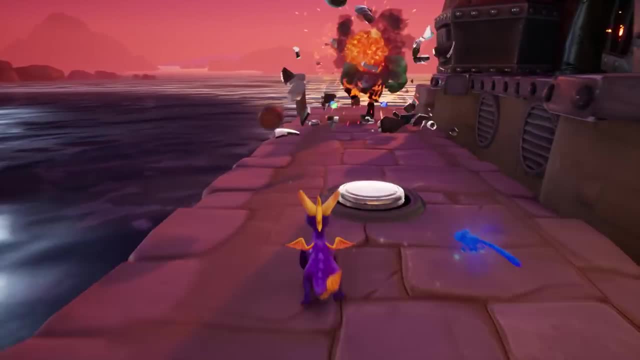 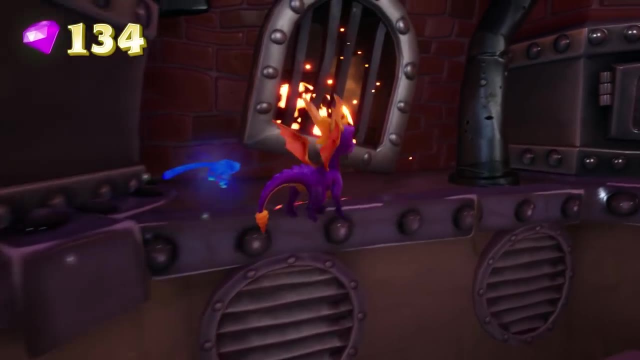 rushed through it. I mean, honestly, I have no problem with you getting this equation wrong, Even getting it wrong with confidence. okay, I've looked like an idiot multiple times in my life, all right, There's no problem with that. 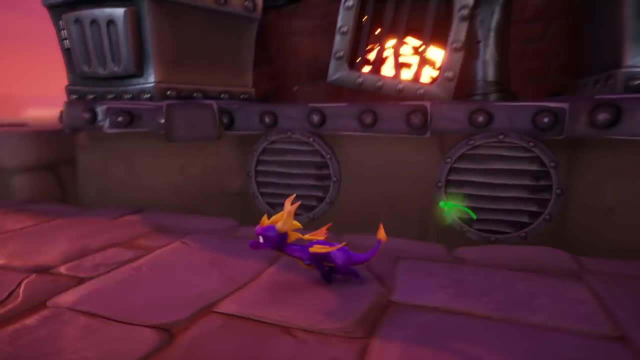 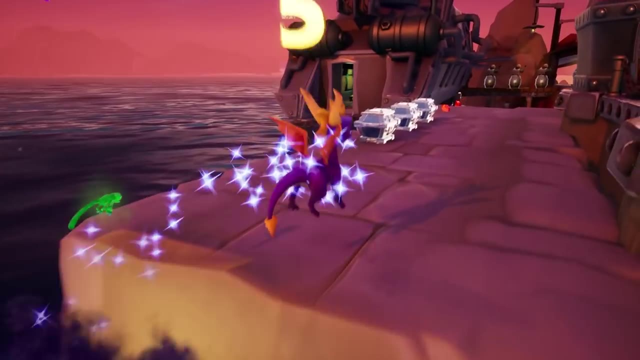 But then, saying that was fun, do another as if. as if you're like the grand authority on math equations or something, when you can't get the simple shit right, dude. And what annoys me is on Twittercom these people are proven right somehow because it's majority wins, you know. 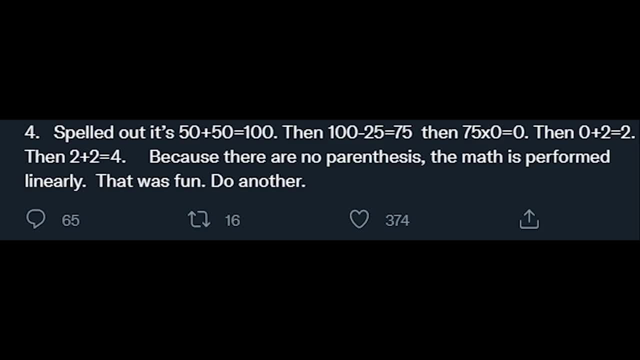 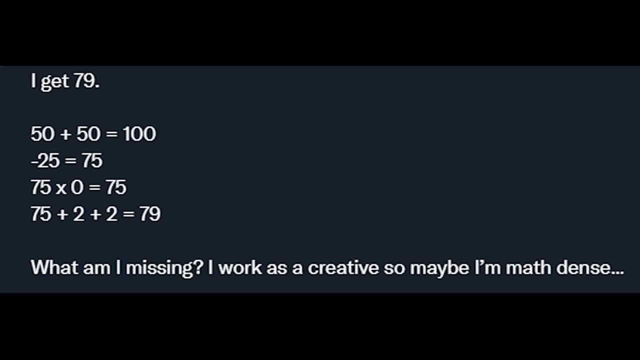 This dude has more likes than replies, so he's like: oh, obviously I'm right Now, don't worry. 4 isn't the only wrong answer. We got a plethora of wrong answers. This person has somehow got 79.. 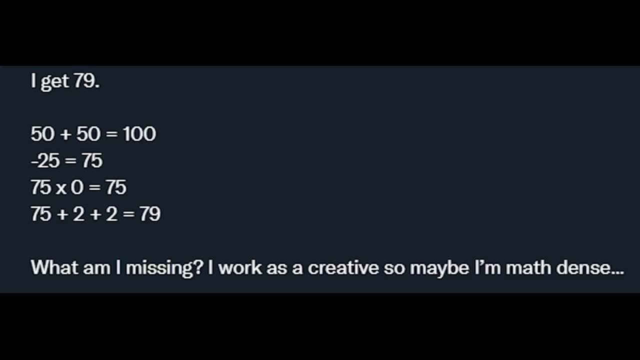 I mean, I'm trying to figure out what mental gymnastics you're doing here, but let's see: 50 plus 50, 100.. Wow, they always start with this one. huh Minus 25, 75.. 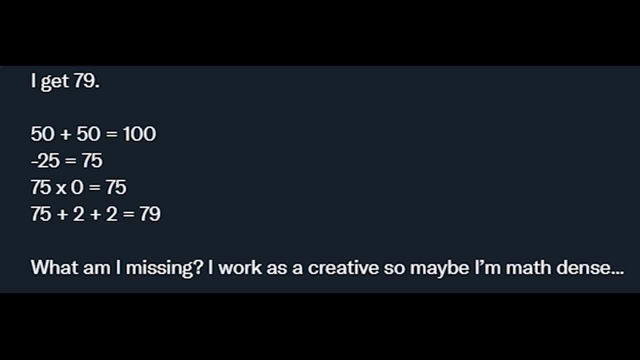 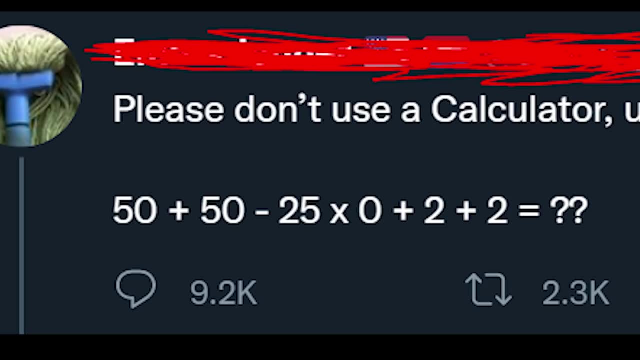 75 times 0, 75.. 75 plus 2 plus 2 is equal to 79.. Wait, I had to glance at the original equation for a second, because this guy's stupidity actually threw me for a loop until I looked at the third one. 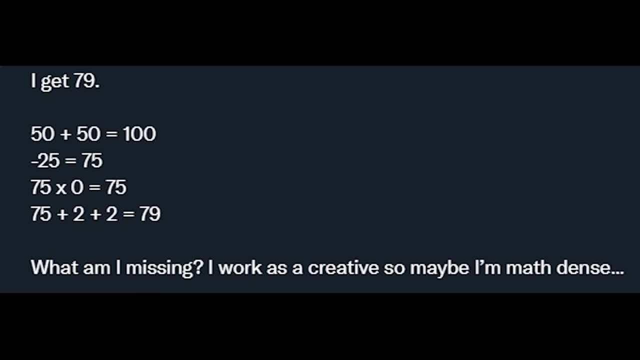 75 times 0 is 75? Dude. I could ask that to a toddler and he would get it right. like: what am I missing? I work as a creative, so maybe I'm math dense, bro. That is no excuse. You can't tell me. I work as a creative, so I don't know what multiplication times 0 does. 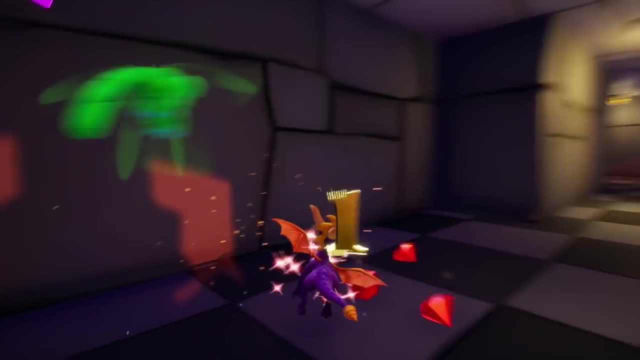 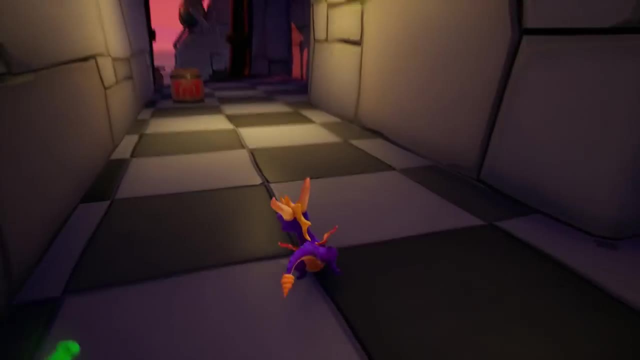 What do you think? just because you're a creative, you have the right to not know basic maths. How are you gonna teach your children? dude, I'm a creative technically, but apparently it is my job to educate morons. on twittercom, This guy said: geez, it's 79.. Why are people getting upset? It's supposed to be fun. 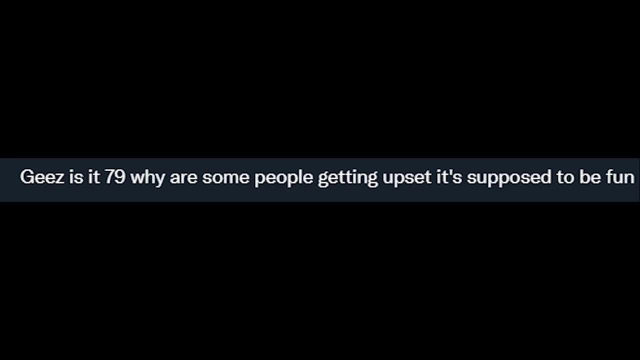 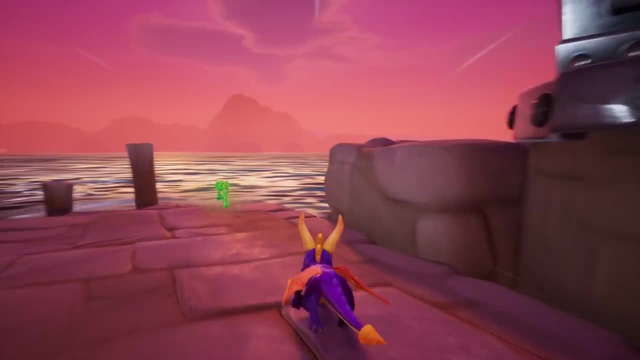 I don't. I don't know a single person who's ever said math is supposed to be fun And the reason people are getting upset is because you're taking something that is objectively a fact and saying it's an opinion Like no, the answer can't be a hundred and four four and seventy nine. 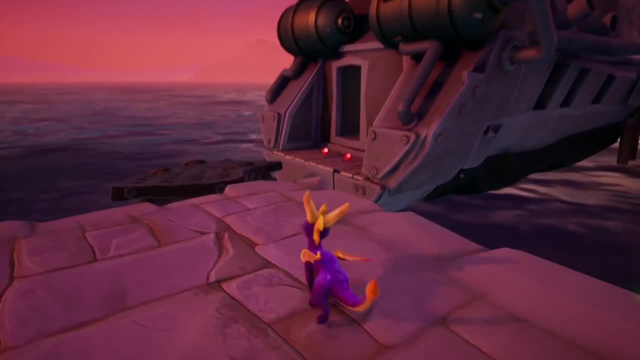 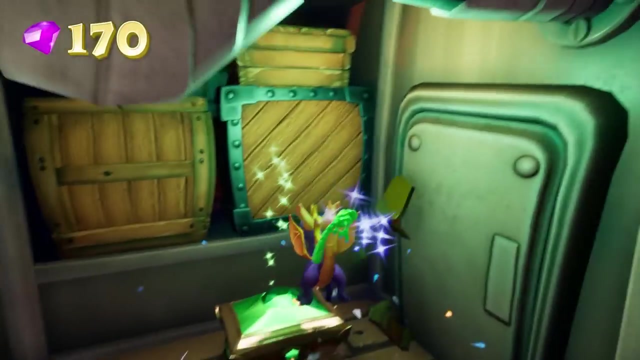 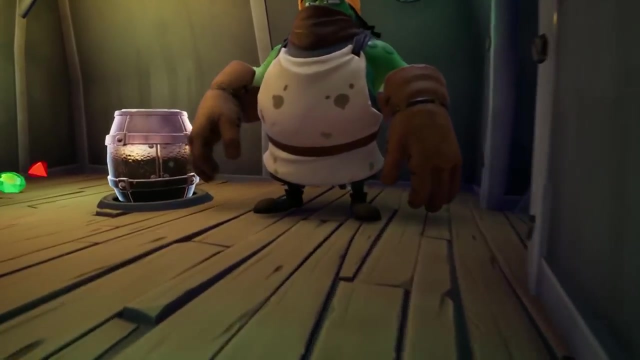 There can only be one answer now. This is different from the situation I was looking at before. there was actually a math equation before which had multiple answers, because People have been taught differently and because the equation itself was not written correctly. It used an outdated symbol that is interpreted differently in renowned universities across the world. 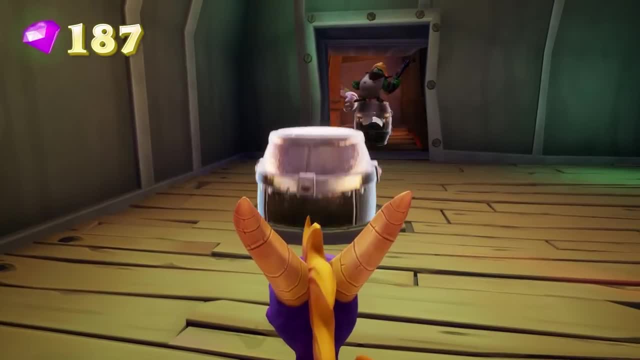 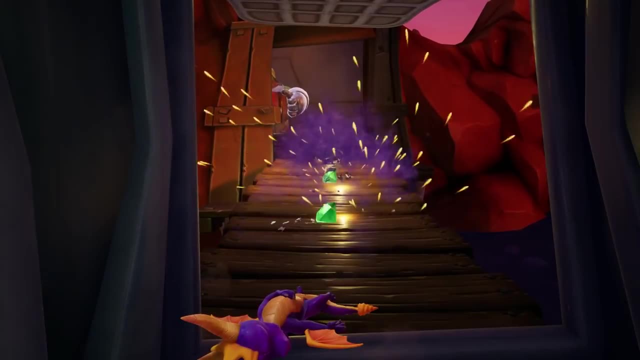 That is the only reason you can have a subjective answer. in maths and in reality There is only an objective answer. but because renowned institutions back it up, Then you are forgiven. But in this case, every single renowned institution, every single high school will tell you only one answer. 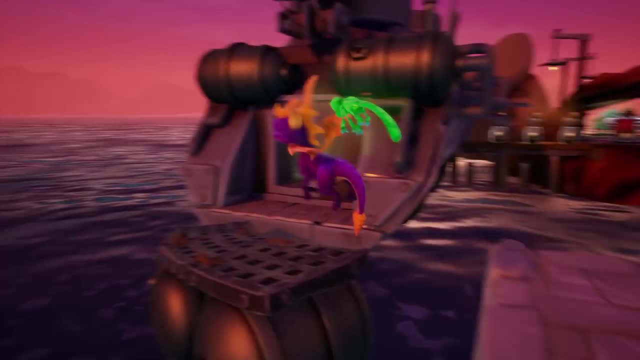 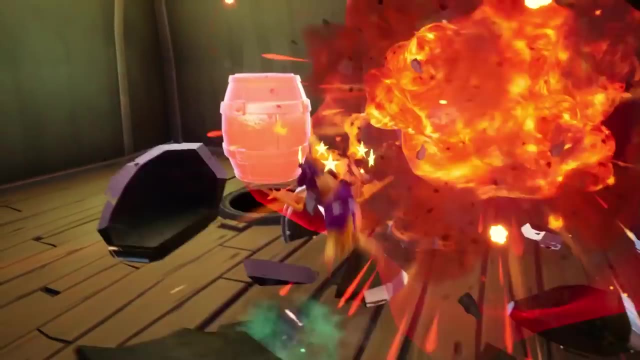 The reason you're getting it wrong Is not because your teacher taught you wrong is because you suck at maths. There's absolutely no way your teacher didn't teach you the order of operations. That's the first thing you learn in mathematics. Now this guy is a new brand of moron. 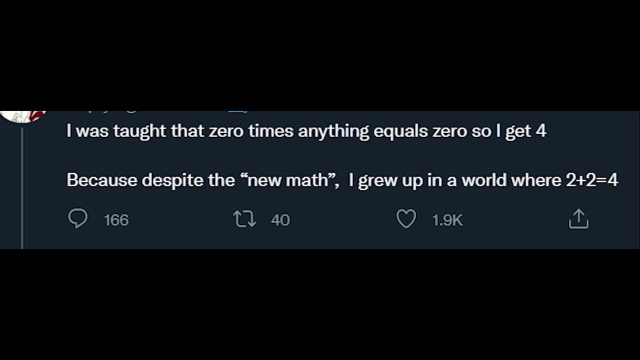 This is like going to the store seeing a new packet of chips on the shelf and being like, oh wow, That's a. that's another kind of stupid that I haven't seen. I was taught that zero times anything equals zero, so I get four. I hate it when you say something that's kind of true, but then still get it wrong. 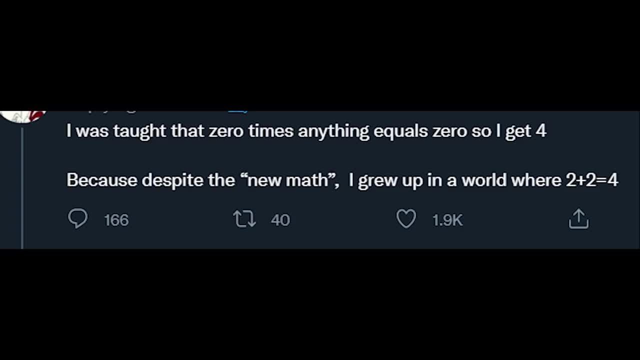 Then he says: Because, despite the new math, I grew up in a world where two plus two is equal to four. So because two plus two is four, your answer is correct. It is two thousand likes, my god. So I'll tell you what this genius is saying pretty much. 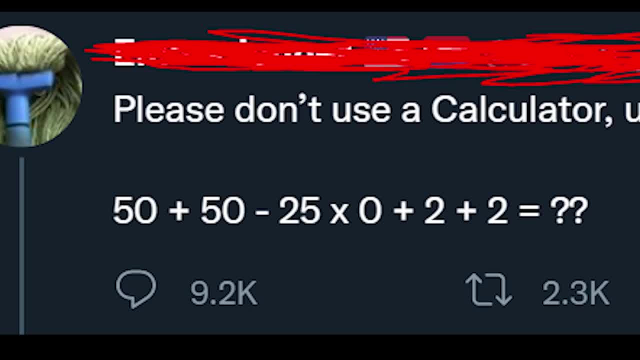 He's saying the first part of the equation, right. fifty plus fifty minus twenty five times zero, that entire thing Translates to zero, and then two plus two is four. therefore, the answer is four. now You would be right if there was a bracket at the very start and right before the multiplication. 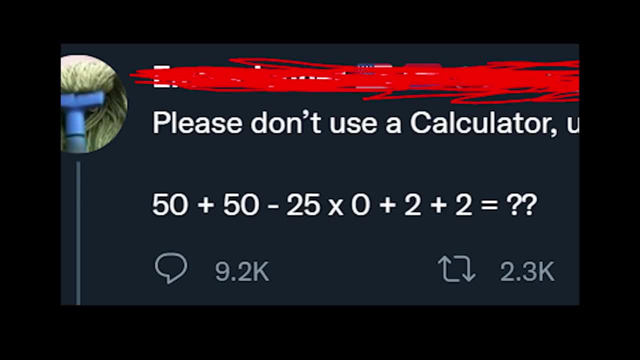 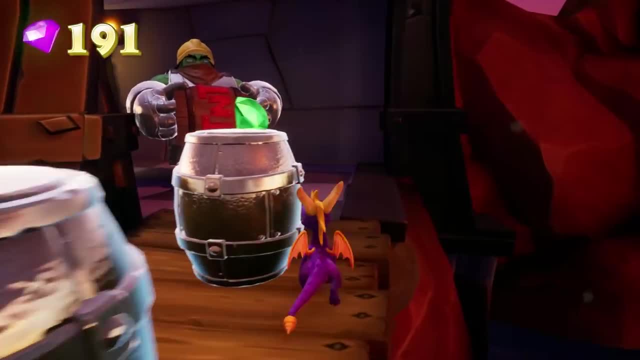 Sign of zero, and then that would result in zero, and then zero plus two plus two is four. So no, the world hasn't changed. This isn't new maths or anything. You're just a complete idiot, dude. What the hell are you saying? new maths? the order of operation has existed for millennia. 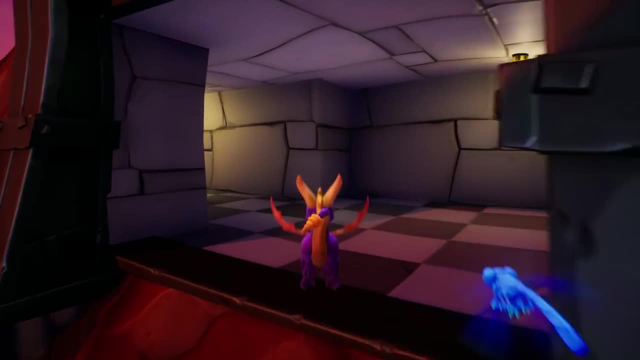 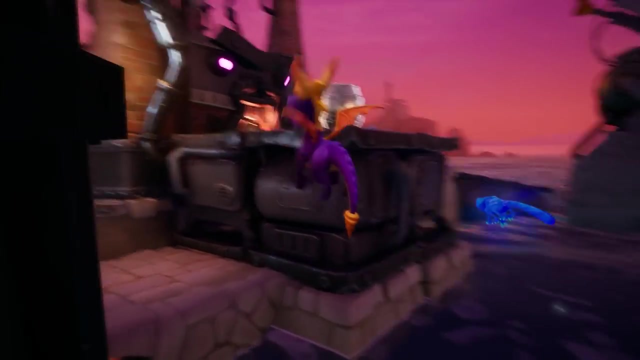 People have been working with equations, using this form of operations, since before you were born. This isn't something new that's randomly come up. I really don't like these people justifying their stupidity by saying: there's new math now. There's one thing to have a completely different. 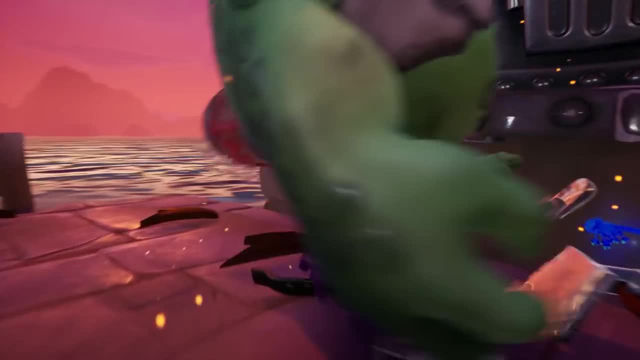 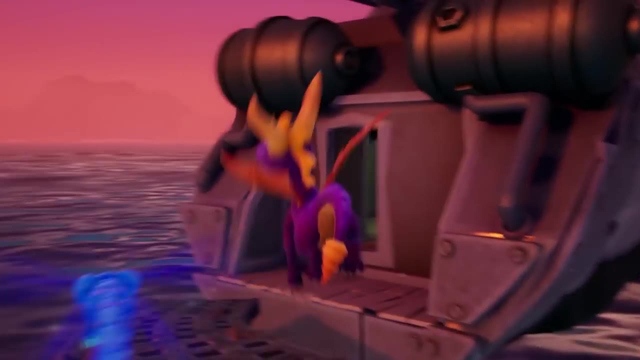 Answer that's wrong. Okay, you know what? I'll excuse all of it. Okay, you can be dumb. you can be dumb all you want, But then don't try to argue with the people who get the right answer, because at that point you're crossing the line. 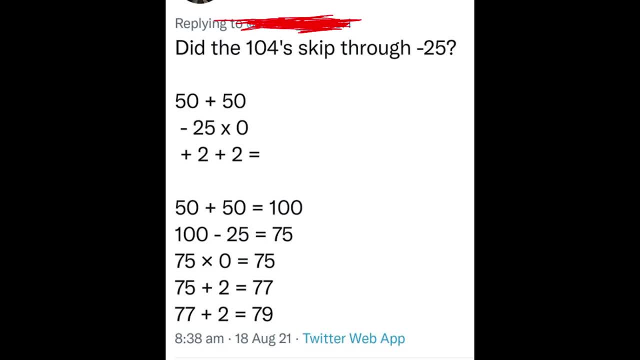 This person says: did the hundred and fours skip through minus twenty five? I assure you we did not. fifty plus fifty minus twenty five, times zero plus two plus two, Fifty plus fifty, a hundred hundred minus twenty five, Seventy five. dude, you don't do addition and subtraction. 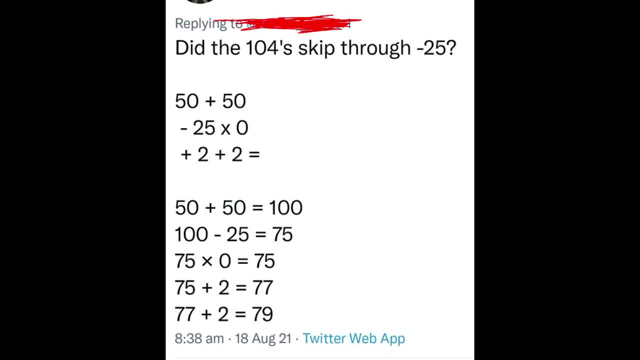 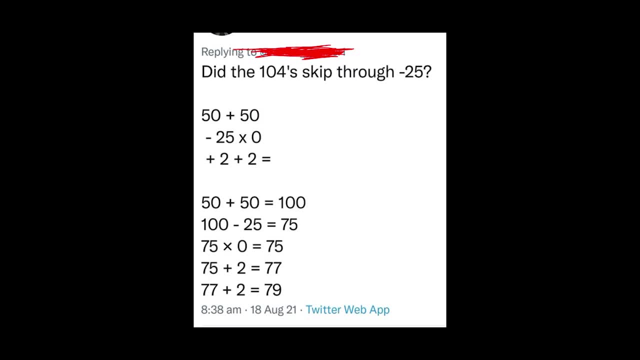 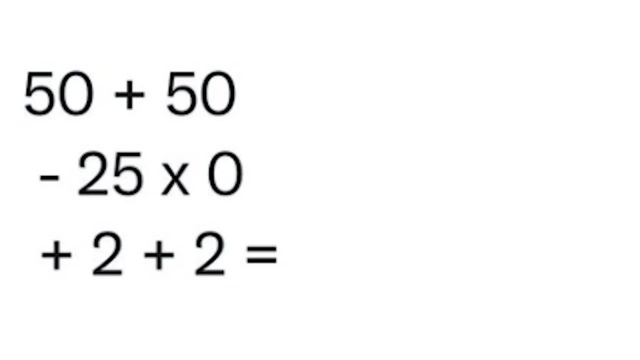 First, you're hurting. you're hurting my brain 75 times zero. seventy five, seventy seven, seventy nine. You know what the dumbest part about all of this is? even in their hypothetical scenario, You don't get a hundred and four by skipping minus twenty five. I'll tell you what you actually get. if you remove the minus twenty five, you get fifty times zero. that is performed first. 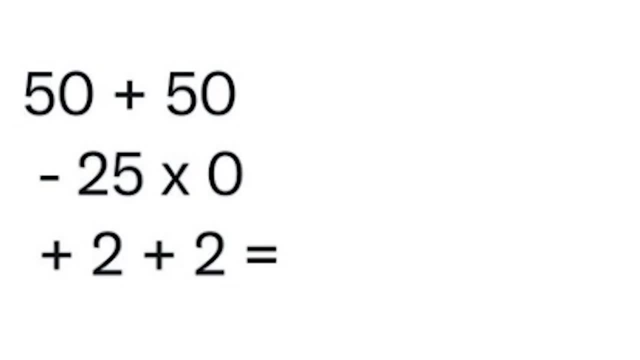 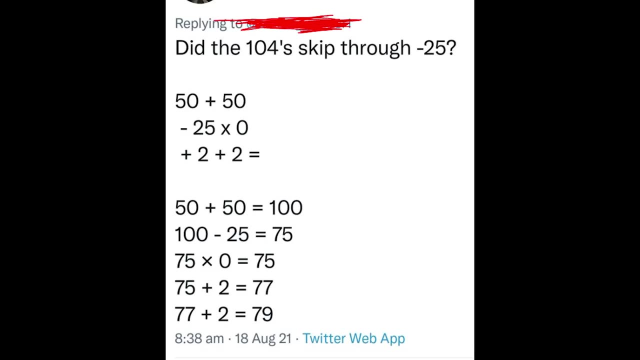 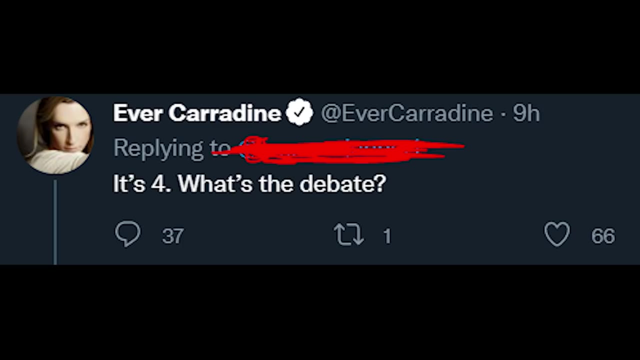 You get zero plus fifty plus two plus two, you get fifty four as the answer. you wouldn't even get a hundred and four. So you're wrong in your dream, Hypothetical world as well. dude, How do you even sleep at night? Here we have somebody who has a verified Twitter check mark saying it's four. What's the debate? 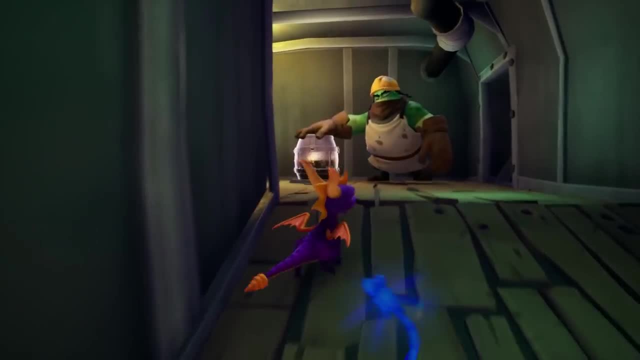 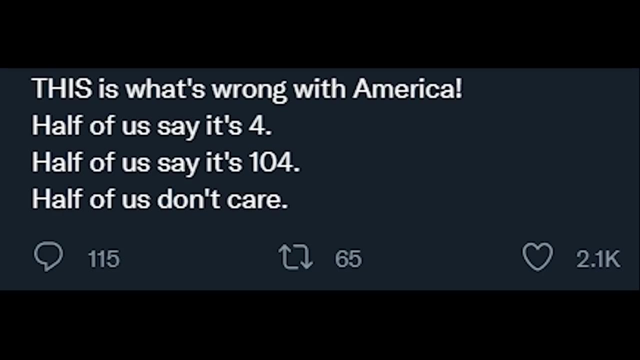 I have no idea who this is, but if you don't know basic maths, I don't think you should be having a check mark. Listen, I feel like there needs to be some sort of boundary basic education. Come on, Somebody made it into an American debate. 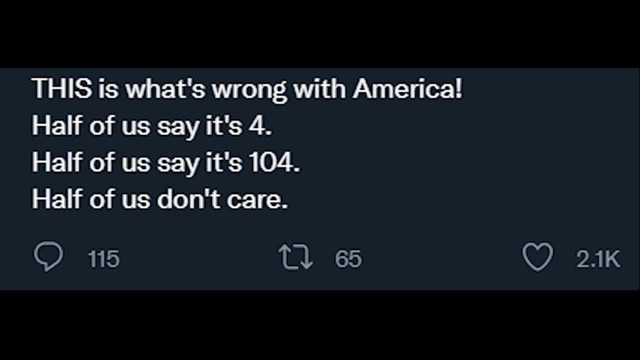 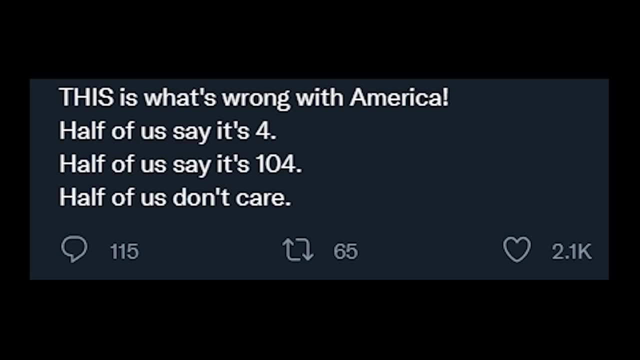 I mean, this is what's wrong with America. half of us say that it's four, half of us say it's a hundred and four. Half of us don't care. I'm gonna be a little Annoying for a second, but because we're talking about maths, there's three halves there, which wouldn't be a half. 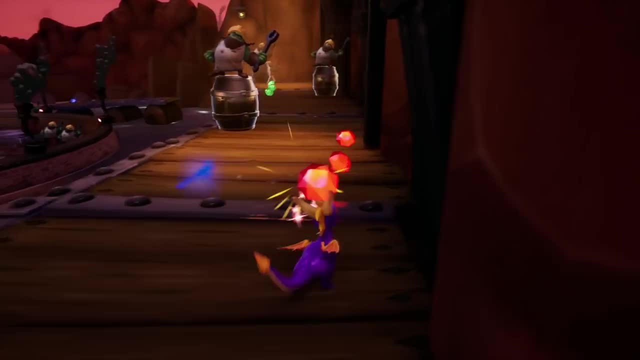 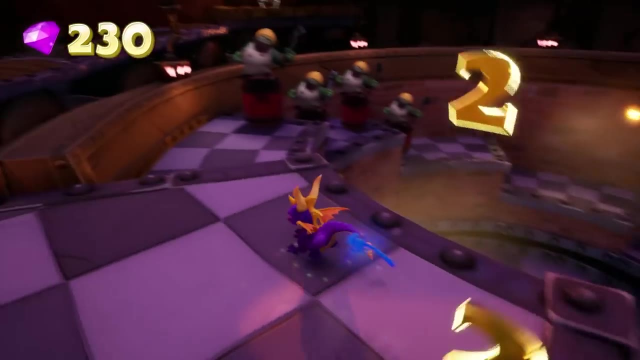 It would technically be a third, but who's counting? but this isn't an issue of America. Okay, this is all around the world, math is the same. Okay, and also, we're all united by Google. if you use the Google calculator, I mean bro, you're gonna get the same answer every time, regardless of location.